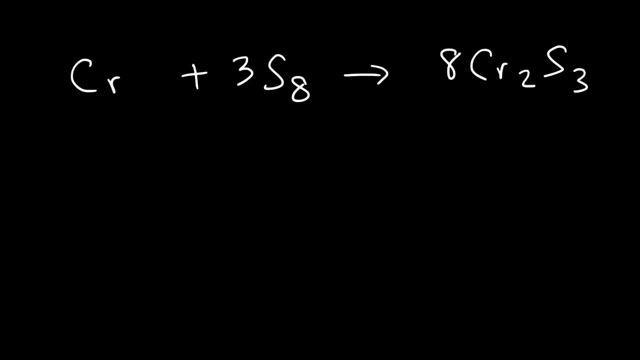 now the number of sulfur atoms are the same on both sides, So now we can move on to balancing the number of chromium atoms. On the right side we have 8 times 2 chromium atoms, Or 16 chromium atoms. So therefore we need to put a 16 in front of Cr. And now 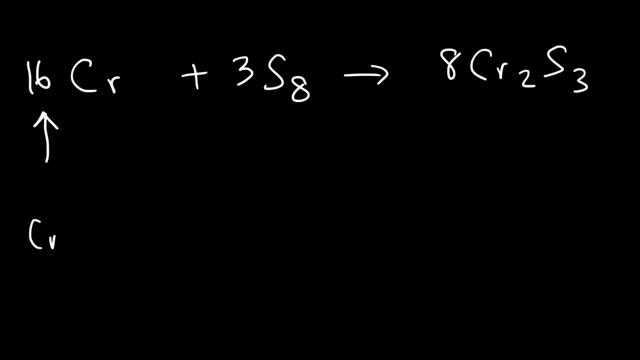 everything is balanced. We have 16 chromium atoms on both sides and 24 sulfur atoms on both sides. Now let's try another example: Mercury oxide, when heated, decompose to elemental mercury and oxygen gas. Feel free to pause the video and work on balancing the equation Now. right now, the 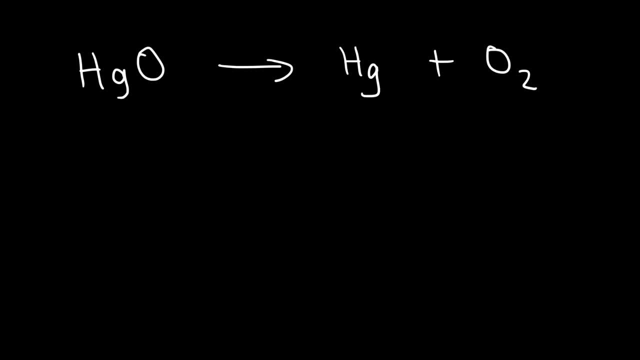 number of mercury atoms are the same on both sides. However, we have two oxygen atoms on the right side and only one on the left side. So in order to have two on both sides, we need to put a two as a coefficient in front of mercury oxide. So 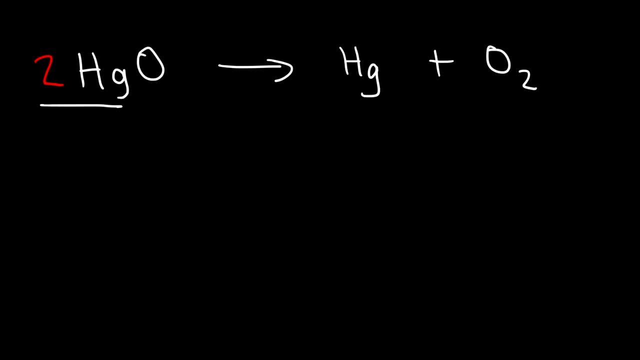 now we have two oxygen atoms on both sides. We got two mercury atoms on the F, only one on the right, So therefore we also need to put a two here, And if you don't see a number, it's the same as having a one in front of it. Now the reaction is balanced. There are 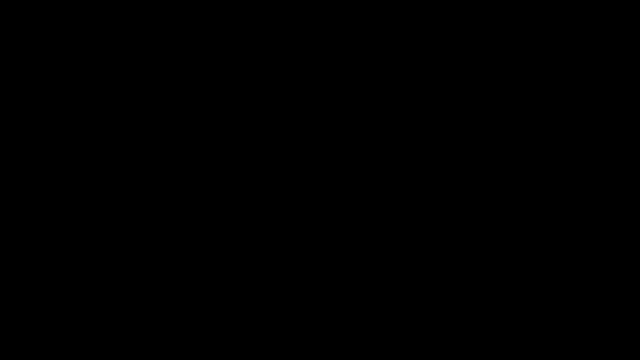 two oxygen atoms on both sides and two mercury atoms on both sides. Now let's look at another example. Aluminum metal reacts with an aqueous solution of copper chloride and it produces an aqueous solution of aluminum chloride plus copper metal. Balance the equation. Now, right now, it 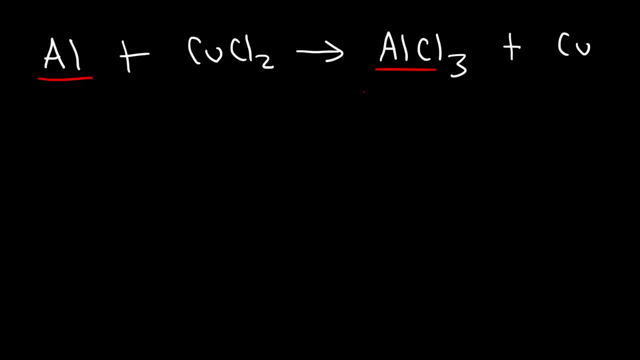 appears as if the aluminum atoms are balanced. They're both one on each side and we have one copper atom on the same side. I mean on each side. However, the number of chlorine atoms is not the same. If we multiply two and three, that's six. So ideally we want to get six chlorine atoms on both sides To do that. 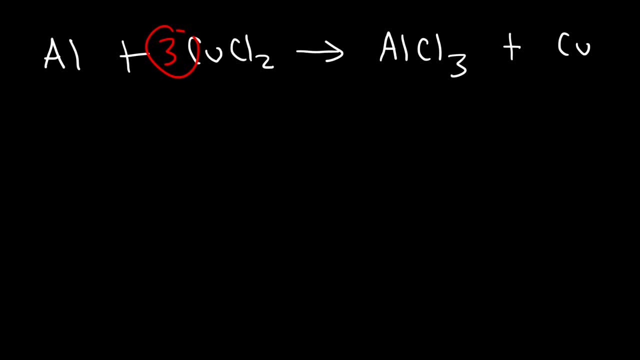 let's put a three in front of copper chloride, because three times two is six. And let's put a two in front of aluminum chloride, because two times three is six. Now the number of chlorine atoms are balanced. So now we have three copper atoms. So let's put a three in front of Cu And we have two aluminum. 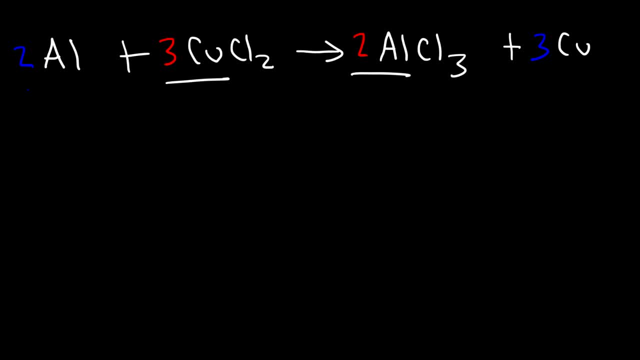 atoms on the right side. So let's put a two in front of Al. Now everything is balanced. Now let's look at another example: Potassium chlorine, when heated, decomposes into potassium chloride plus oxygen gas. Go ahead and balance the chemical equation. Right now we have one potassium 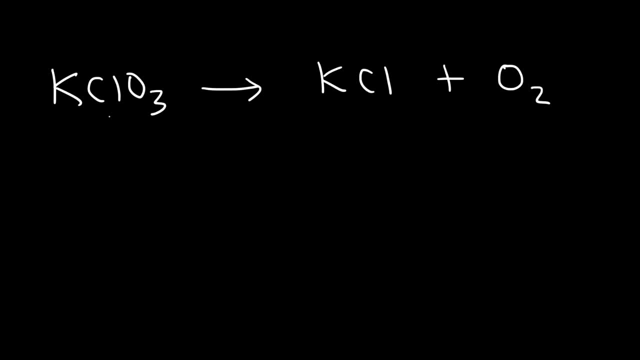 atom on both sides and the number of chlorine atoms are the same on both sides. The only thing that's different is the number of oxygen atoms. So two times three is six. Therefore, we want to get six oxygen atoms on both sides. So let's start by putting the two in. 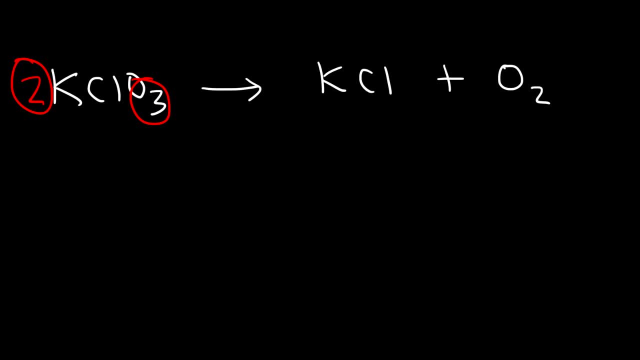 front of KClO3, because two times three is six, And let's put a three in front of�� front of O2.. So now we have six oxygen atoms on both sides. Now notice that we have a 2 in front of K and Cl. Therefore we need to put a 2 in front of KCl Now. 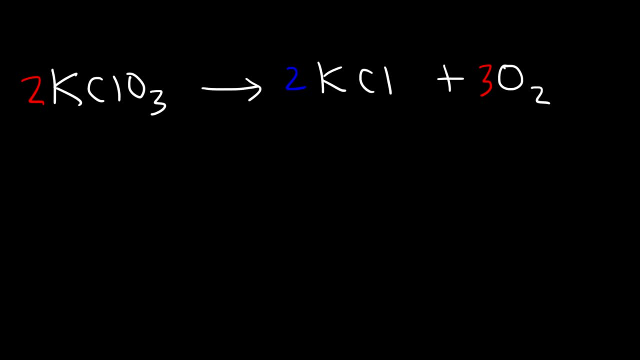 everything is balanced. So this example wasn't that difficult and some problems will not be. Others will be harder. Now let's look at another example. Let's say if we have C3H8, propane reacting with oxygen gas, producing carbon dioxide plus. 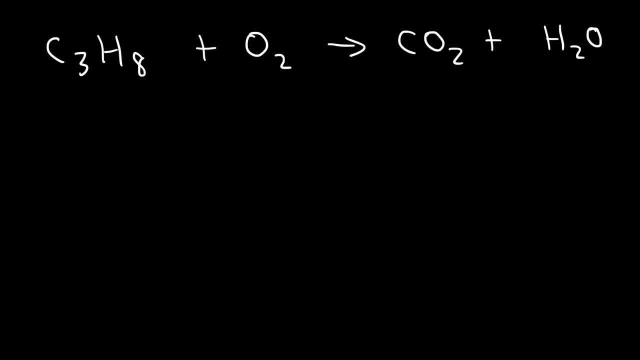 water. So this is a combustion reaction. It's very exothermic, It generates a lot of heat. Let's balance the equation Now. when dealing with combustion reactions, personally I prefer to balance the carbon atoms first. There are three carbon atoms on the left, but only one on the right, So therefore I need to put a. 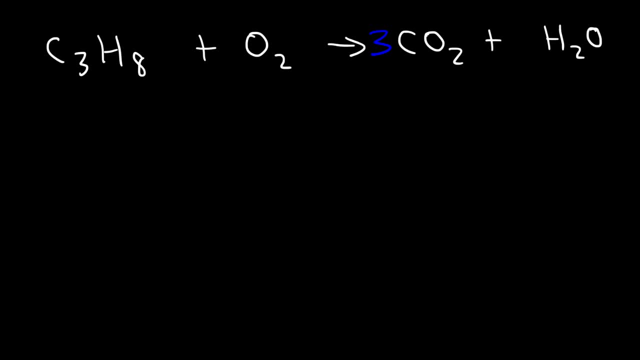 3 in front of Cl2Cl, So that I can have three carbons on both sides. Next I'd like to move on to the number of hydrogen atoms. I have 8 on the left, only 2 on the right, So to get 8 on. 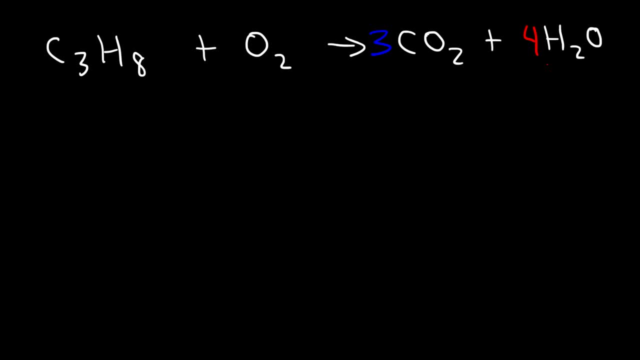 both sides. I need to put a 4 in front of H2O, because 4 times 2 is 8.. Now the last thing that I like to balance for combustion reactions is the number of oxygen atoms On the right side. 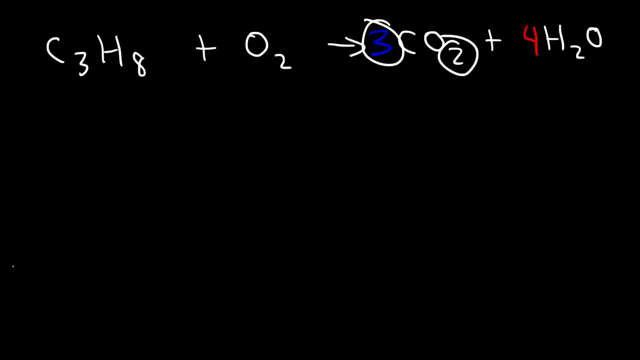 we have six oxygen atoms from the three CO2 molecules, because 3 times 2 is 6. And 4 times 1 is 4, so we have four oxygen atoms from the four water molecules. So therefore we have a total of 10 oxygen atoms on the right side. So what number do? 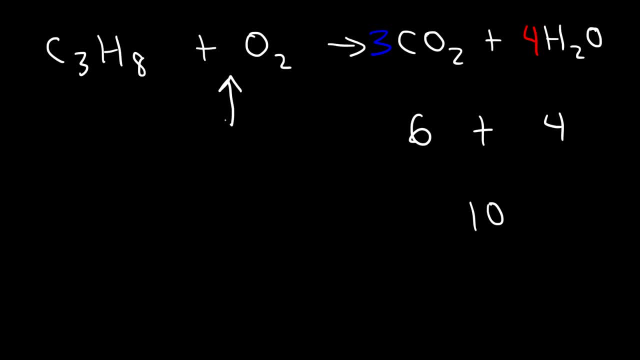 we need to put in front of O2 to get 10 oxygens as well. Well, 10 divided by 2 is 5.. So we need to put a 5 in front of O2, and now the reaction is balanced. 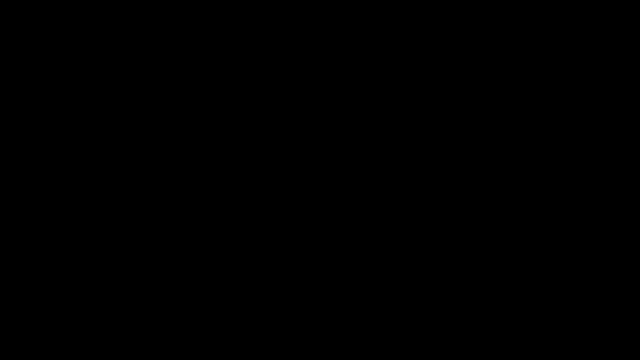 Let's try another combustion reaction. So let's say, if we have ethanol C2H5OH plus O2, and it produces carbon dioxide and water, So we have another combustion reaction, Feel free to try this one. So there are two carbon atoms on the left. so 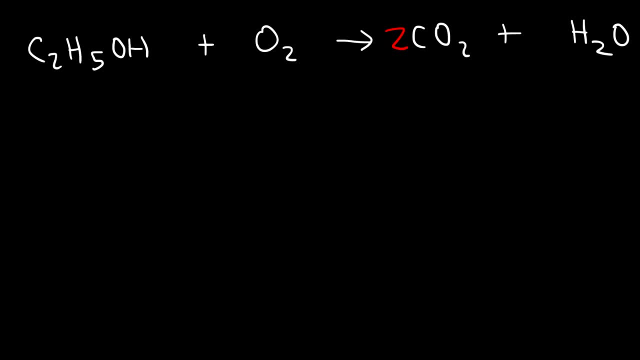 therefore, I need to put a 2 in front of CO2, so I can have two carbon atoms on the right side. Now let's move onto the number of hydrogen atoms. I have 5 plus 1, or 6 hydrogen atoms on the left side, So I need 6 on the right, 6 divided by 2,. 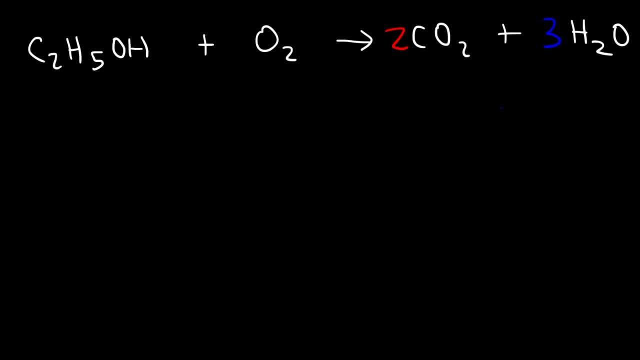 that's 3.. So let's put a 3 in front of H2O. Now the last thing that we need to balance is the number of oxygen atoms. So we have four oxygen atoms from the two CO2 molecules. 2 times 2 is 4. And we 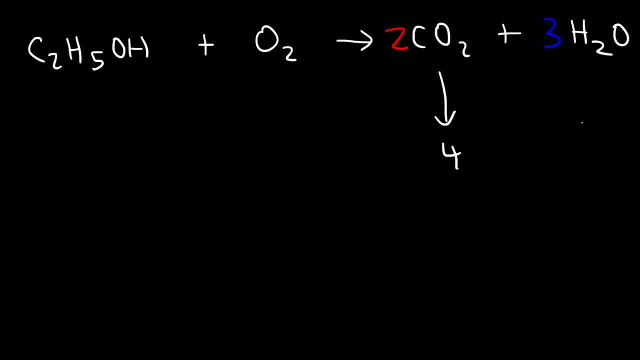 have three oxygen atoms from the three water molecules, And 4 plus 3 is 7.. Now I already have one oxygen atom in ethanol, so to get a total of 7 on the left side I need 6 more, And 6 divided by 2 is 3, so therefore I need a 3 in front of O2.. 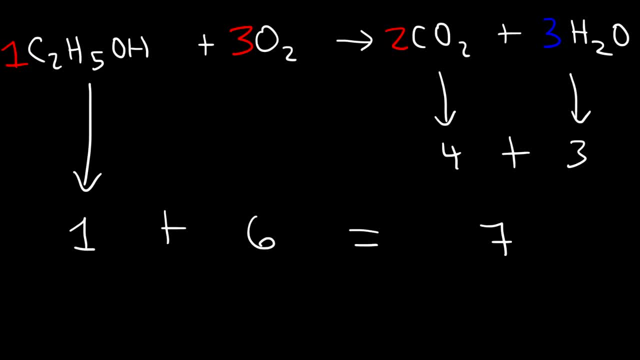 And this reaction is now balanced. Let's try a harder example. Ammonia reacts with oxygen gas to produce nitrogen monoxide and water. Go ahead and balance the reaction. So the number of nitrogen and oxygen atoms are currently the same on both sides. The only thing that's different is the hydrogen atom. So we 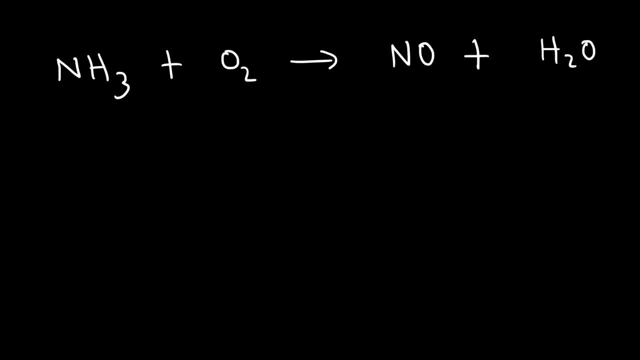 have three on the left, two on the right. So we have three on the left, two on the right. So we have three on the left, two on the right. So 2 times 3 is 6.. Let's try to get six hydrogen atoms on both sides. So 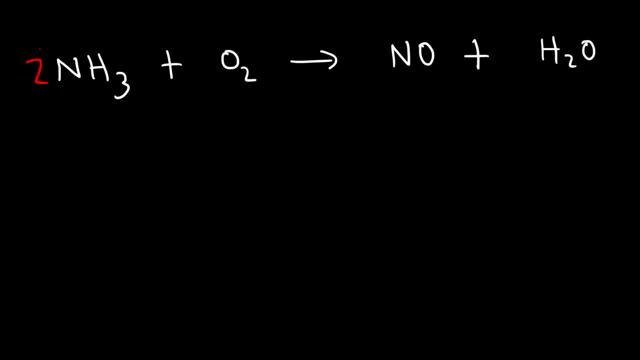 therefore we need to put a 2 in front of NH3, because 2 times 3 is 6. And we need a 3 in front of H2O. So now we have six hydrogen atoms on both sides. Now we have two nitrogen atoms on the left but only one on the right. So therefore we 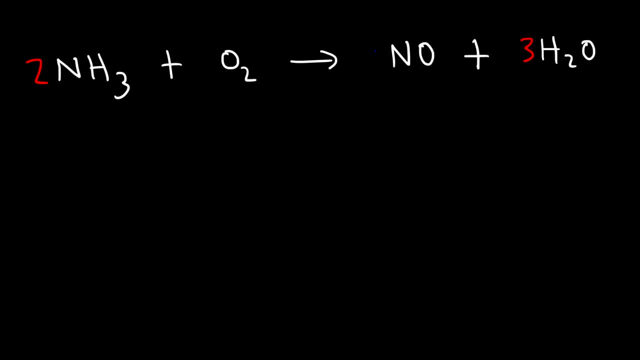 need to put a 2 in front of NO, So now the number of hydrogen atoms and nitrogen atoms are equal. So now let's move on to the oxygen atoms. We got 2 from NO, 3 from water, so that's a total. 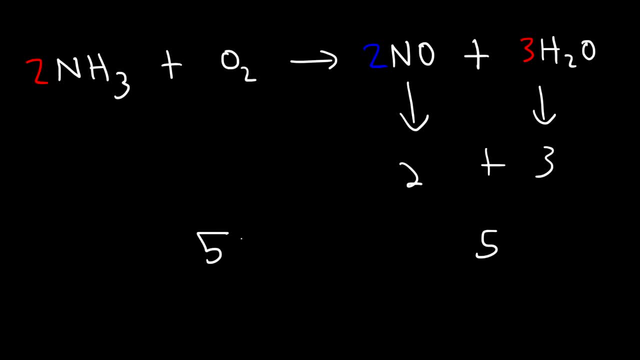 of 5.. Now we need 5 on the left. 5 divided by 2 is 5 over 2.. That's a fraction which is the same as 2.5.. Now, if you get a fraction, it's not the end of the world. You just simply. 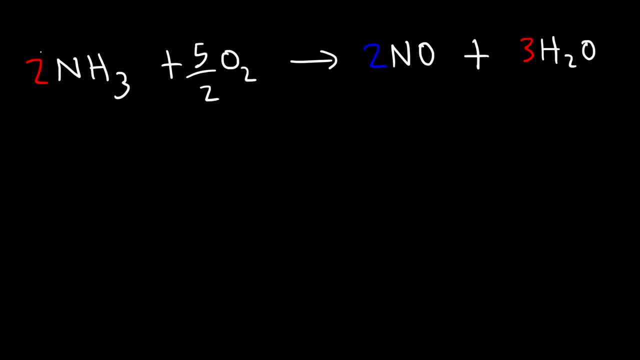 need to know what to do. You want to get a whole number, So what I'm going to do is multiply everything by 2.. Whatever this denominator is of the fraction, multiply by that number to get rid of the fraction. So 2 times 2, that's 4.. So in 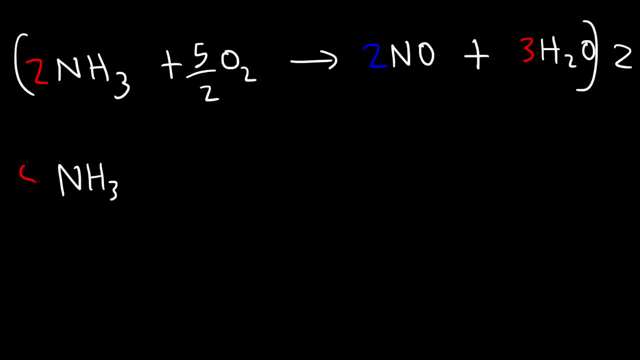 front of NH3, I now need a 4.. Now, if you multiply 5 divided by 2 by 2, the 2's will cancel, leaving you with a coefficient of 5.. Now I'm going to multiply NO by 2, so we're going to have 4 NO molecules instead of 2.